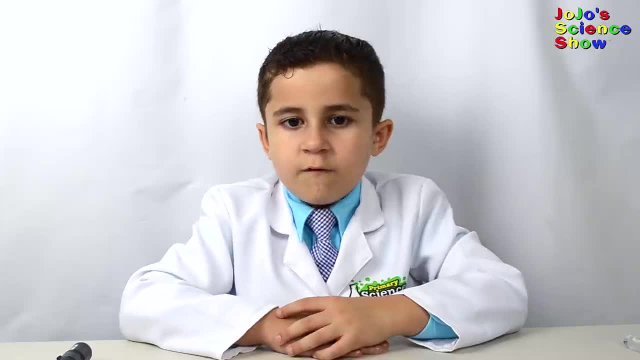 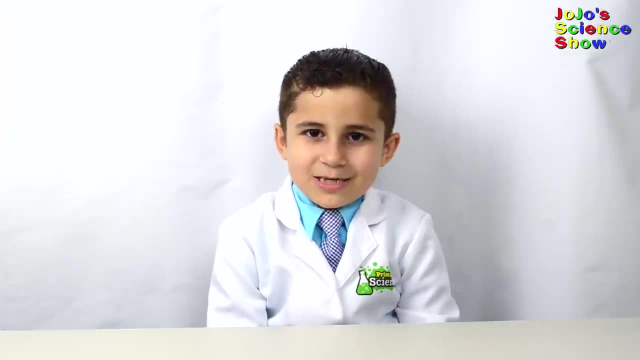 This is when light reflects off the aerosol droplets. This is when light reflects off the aerosol droplets And since light comes from a reflection to glass over and over and comes out the other side, You can use total internal reflections to send messages in different colors and flashing lights. 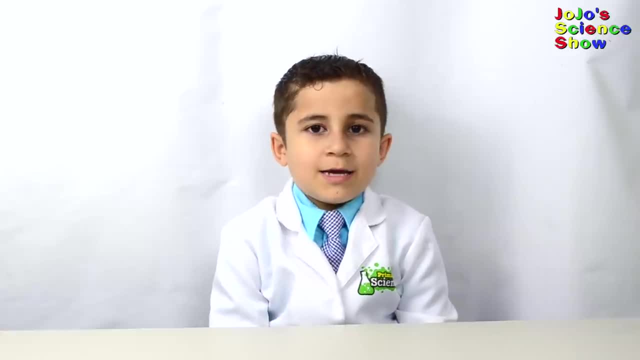 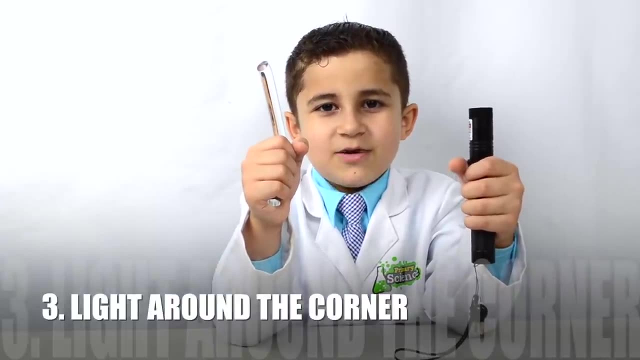 from one end of the rod or fiber to the other end. This is how fiber optics that bring the Internet to your house works. For the next experiment, you'll need a bent acrylic rod and laser pointer. Do the same for the second experiment. 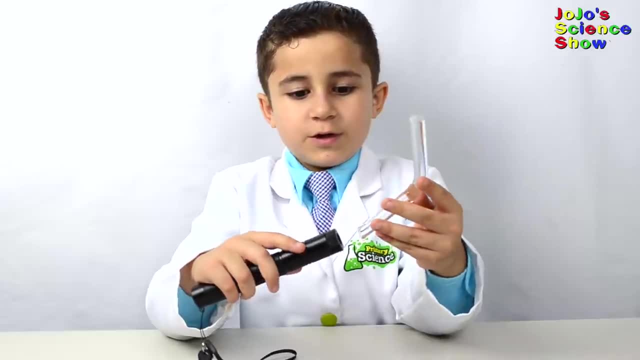 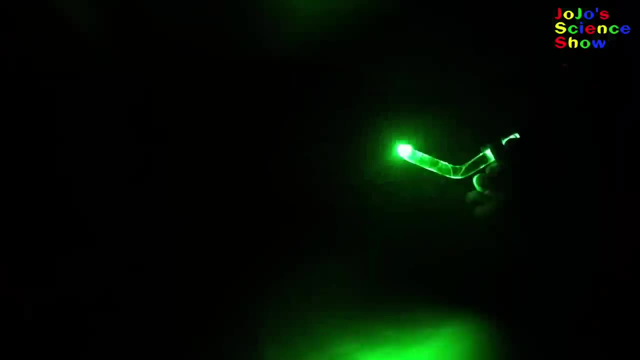 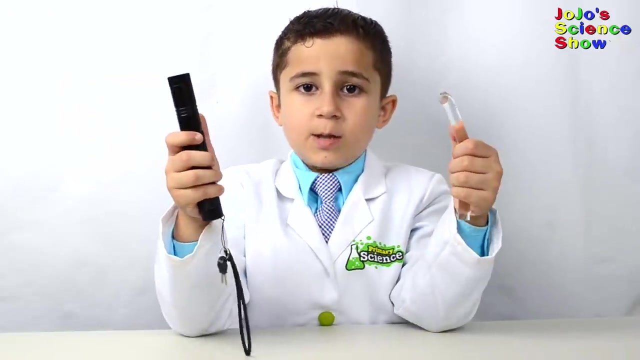 Let's see if we can make the light travel around corners. The light is bouncing back and forth And going around the corner And coming out the other side. Oh wow, it works. The light travels around the corner and comes out the other side of the rod. 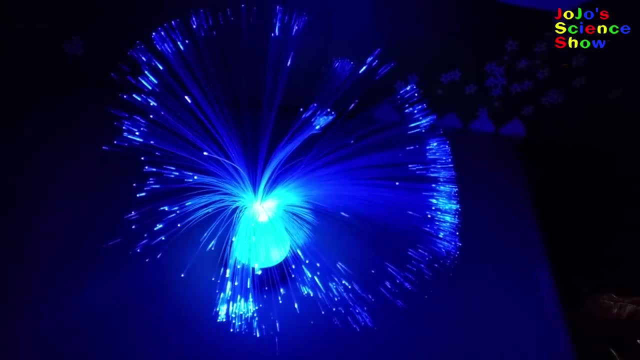 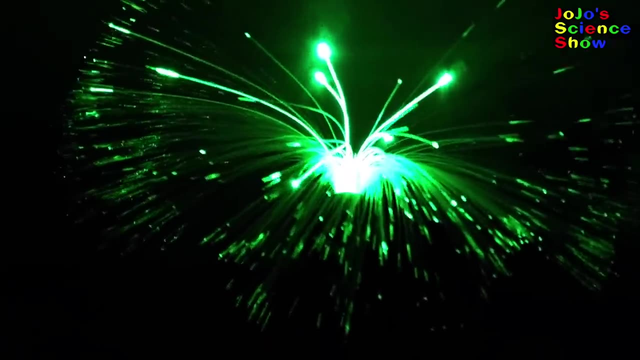 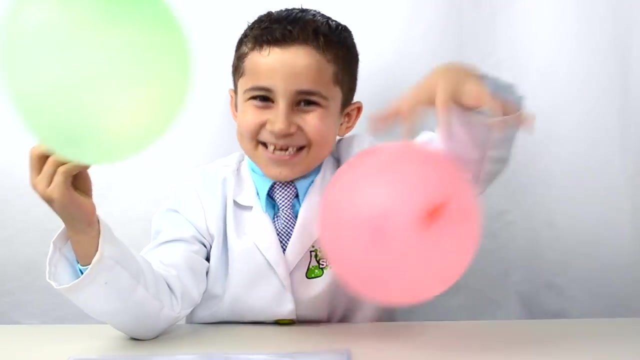 As long as the angle is not too much. This decoration is an example of total internal reflection. See how the light is going around the bend. Doesn't that look really nice? For our next experiment, we'll use light to pop balloons. We will need a frontal lens and some balloons. 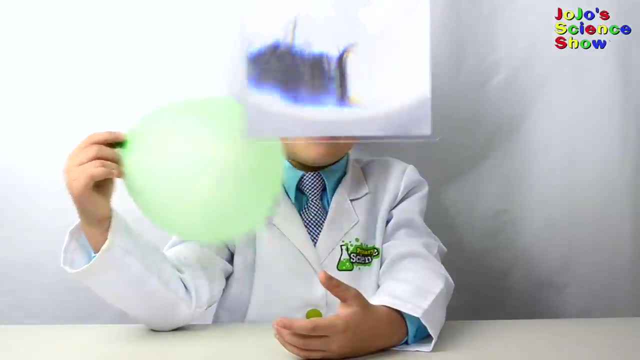 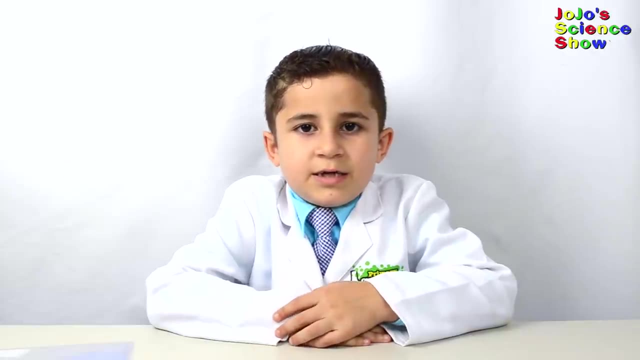 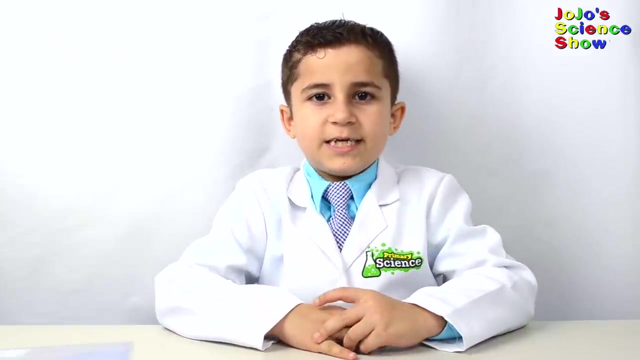 A frontal lens is like a big magnifying glass. It's really cool. Light is awesome, isn't it? A frontal lens causes light rays to bend and you can use it to focus all these light rays on one point. When all the light rays focus on one point, the light energy turns to heat. 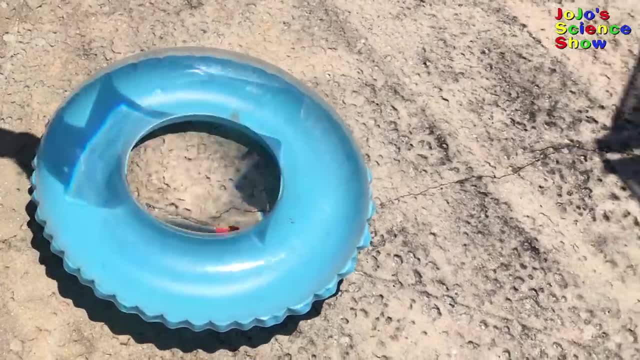 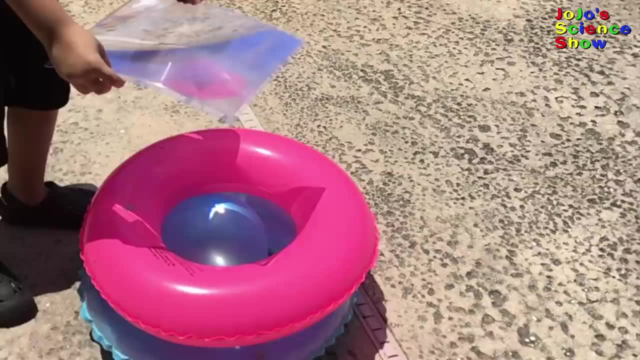 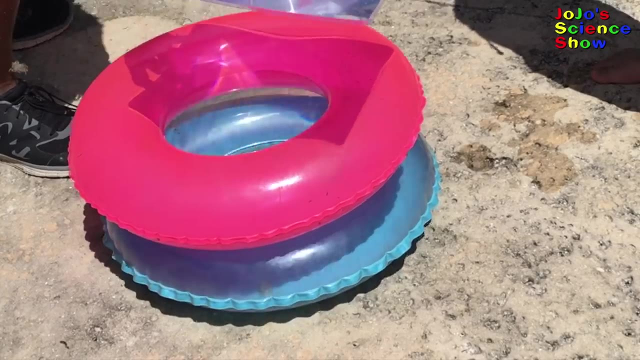 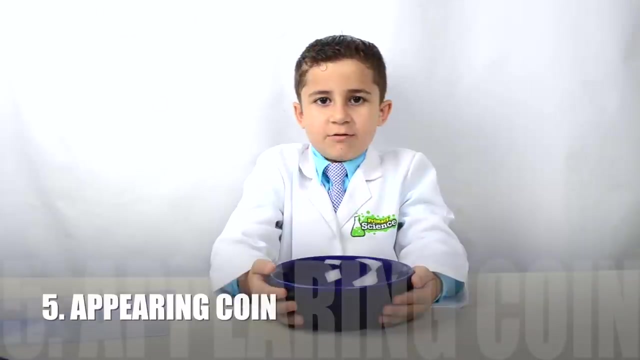 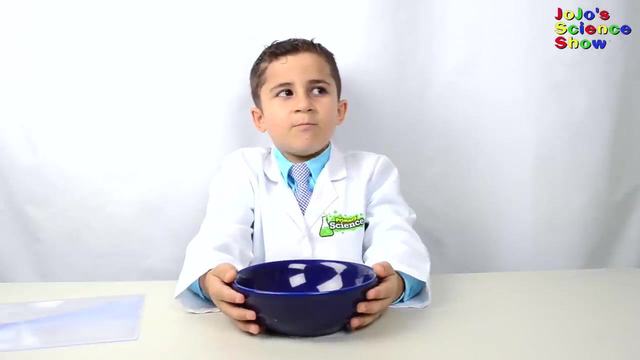 We can use it to pop all these balloons. This next experiment is called a peering coin. You'll need a bowl, a coin and some water, As we can see more like can't see. this coin is in the bowl and you can't see it. 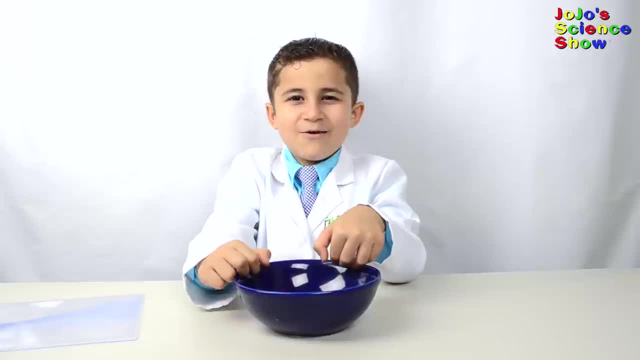 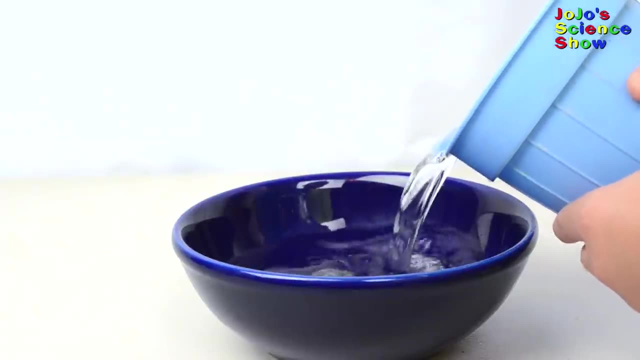 But when we pour water in the bowl, prepare to be amazed. Before I poured the water, you couldn't see the coin. When I poured the water in, you couldn't see the coin. When I poured the water in, the coin appeared. 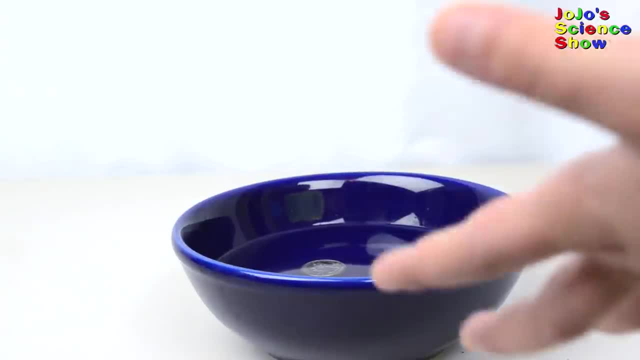 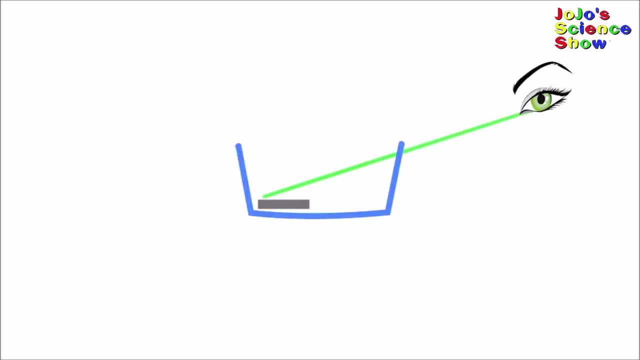 That's because water bends light. When the light bends, it allows your eyes to see into the bowl. We can't see the coin because the side of the bowl is blocking the light from reaching our eyes. But when there is water, it bends the light so that we can see the coin. 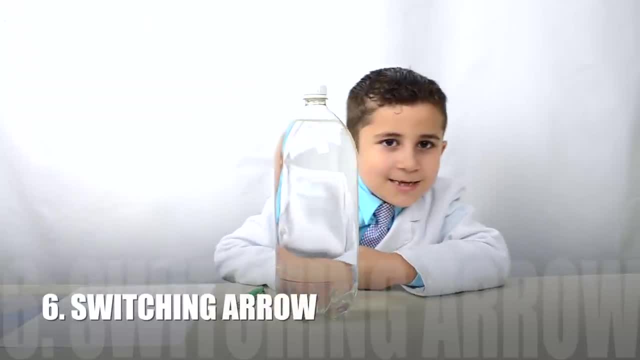 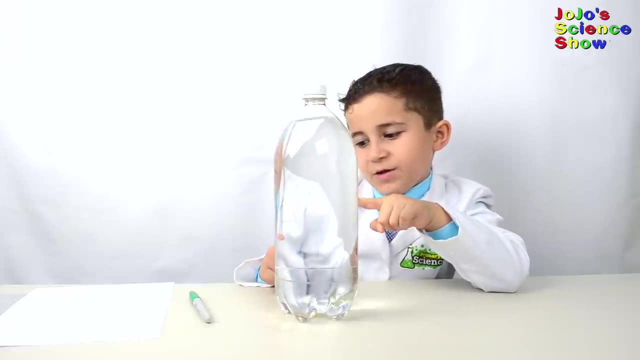 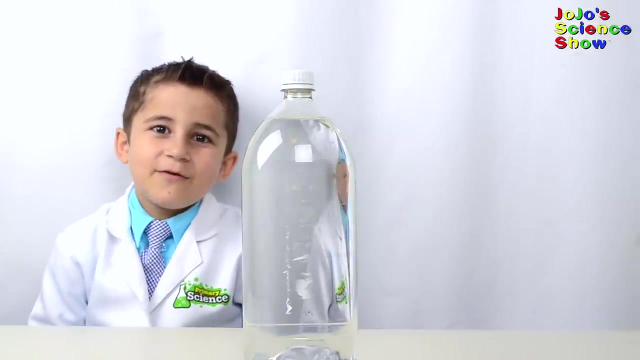 This is called refraction. This experiment is called the switching arrow. How funny do I look For this experiment? you'll need a bottle filled with water, A marker and a piece of paper. This is a fun trick to play on your friends. Prepare to be. 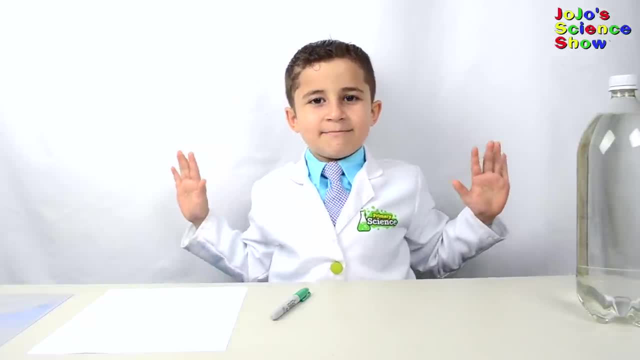 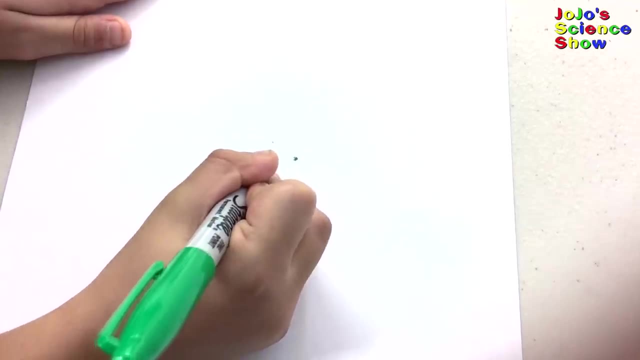 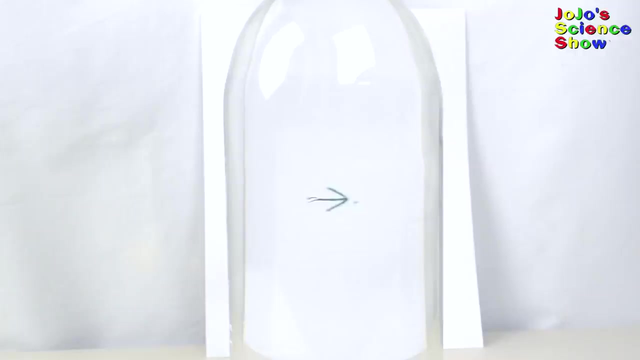 amazed again. Can you wait? Maybe some of you can't wait, So so you just draw an arrow. First, draw an arrow on your paper. Which way is the arrow pointing, Are you sure, Whoa? So what makes the arrow switch? The bottle is in the middle, The water in the 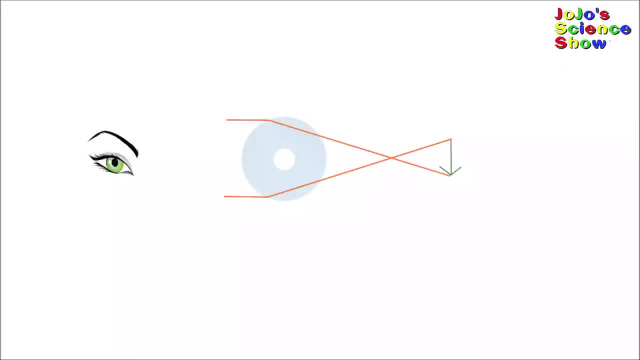 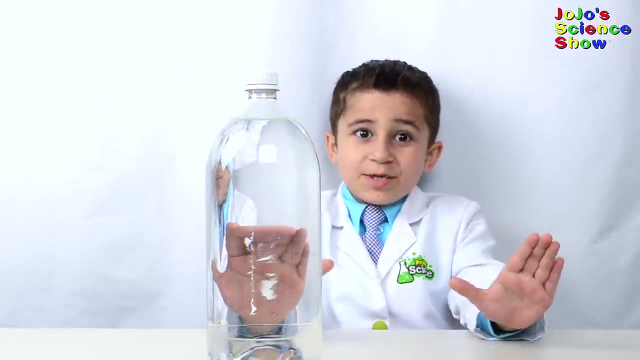 bottle bends the light. It acts like a convex lens or a magnifying glass. Where the light crosses is called the focal point. Because the arrow is behind the focal point, it gets reversed As the light travels to our eyes. Look, I have two left hands. Wait, That's. 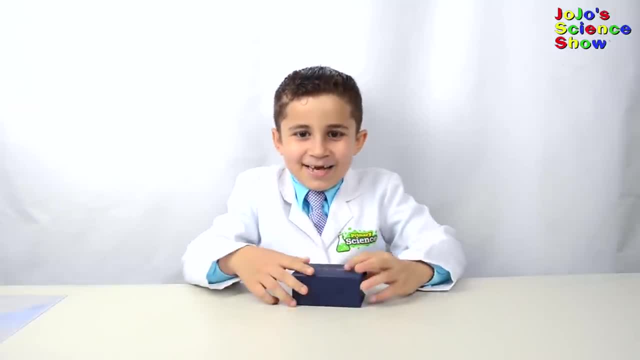 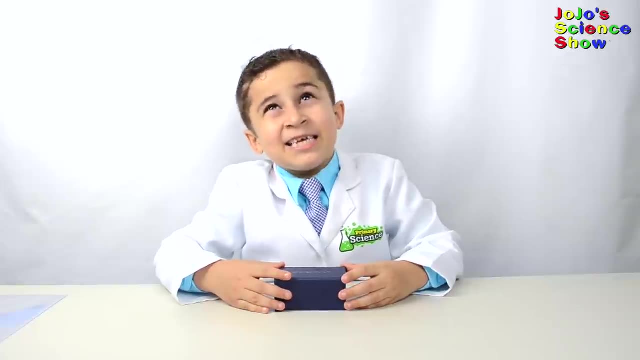 impossible. Do you want to see what's in this box? What's inside this box will help us to make a rainbow. Now you might think that's crazy. It's a glass prism. Now, be careful with this. You can't get these. 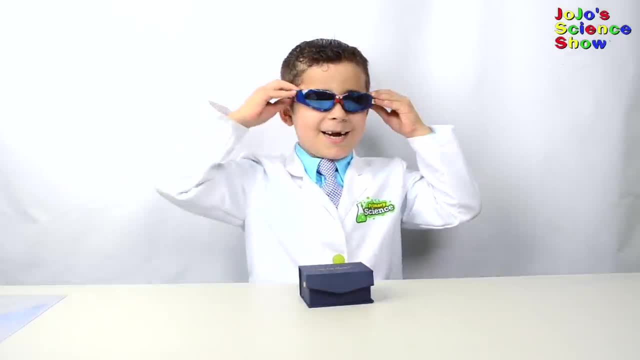 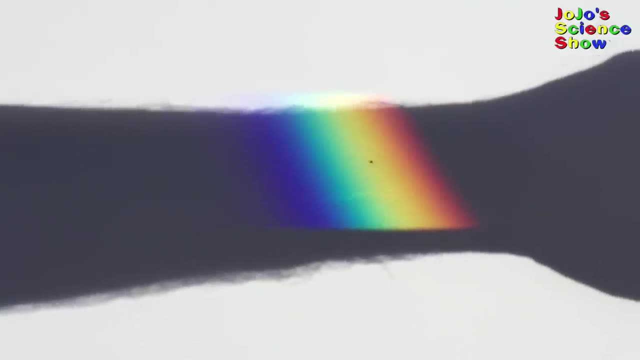 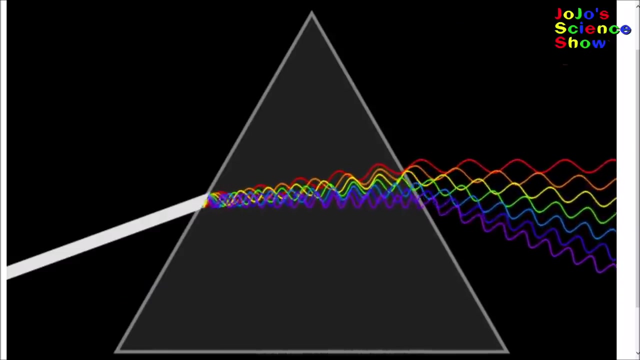 prisms dirty. Now we have to go out in the sun. All you need is some sunscreen And that prism. Let's see, Wow. The prism is splitting the white light into all the colors of the rainbow. The light travels slower in the prism, causing the white 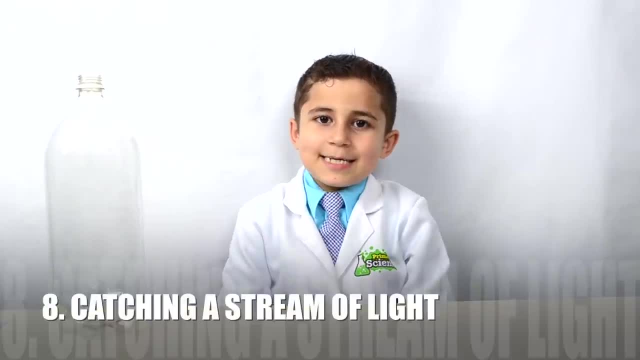 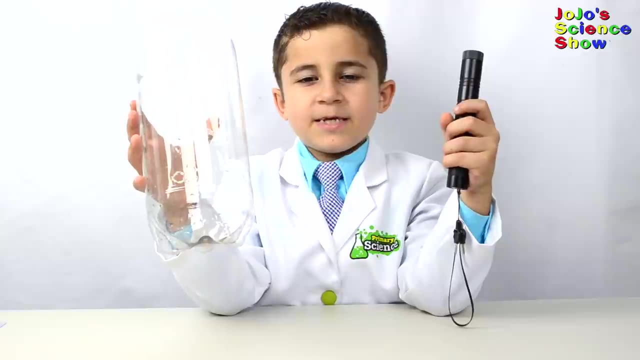 light to split into all the colors. This next experiment is called streaming light. You'll need a bottle with a small hole in it and a laser pointer. This experiment is about total internal reflection with a stream of water. You'll need to go over your kitchen table. You'll need to go over your kitchen table. You'll need to go over your kitchen table. You'll need to go over your. 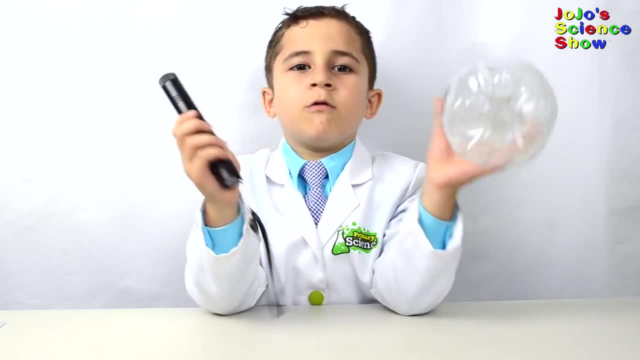 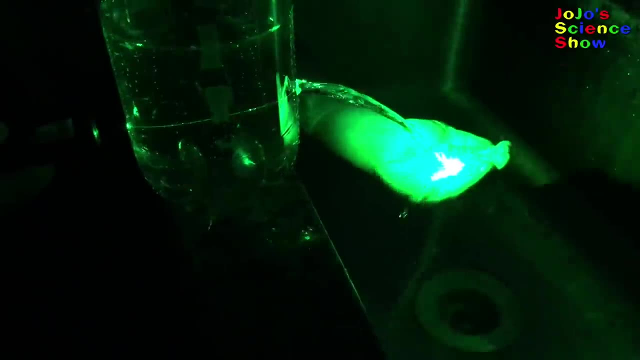 kitchen sink, or in your backyard, or in a very big bowl or something like that. So point the laser through the hole in the bottle. Do you see how the light is following through the stream of water? And I'm catching the light with my hand. 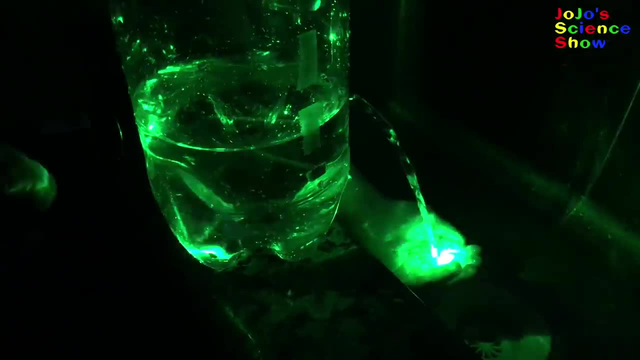 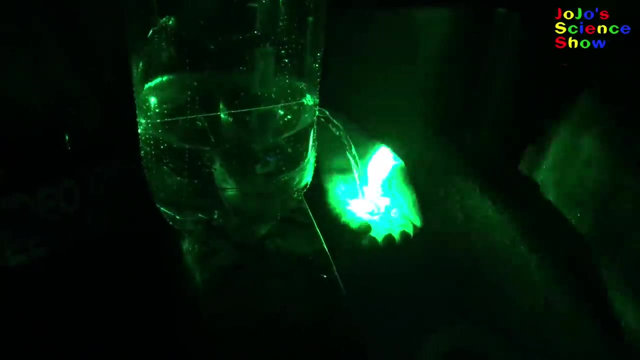 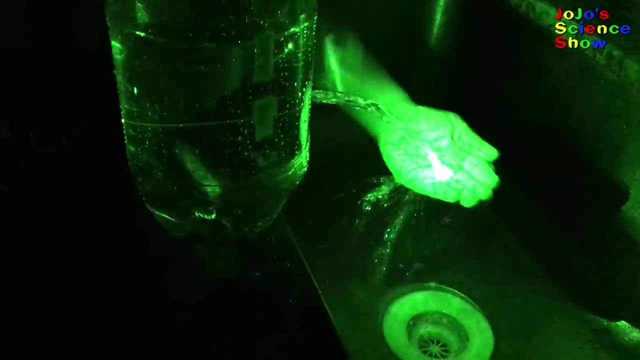 That's awesome. Total internal reflection also works in a stream of water. Who knew I'm really catching a lot of light here. It's kind of tricky to get the laser in the right spot. This is called a photoresistor. We're gonna use it in our next experiment. A. 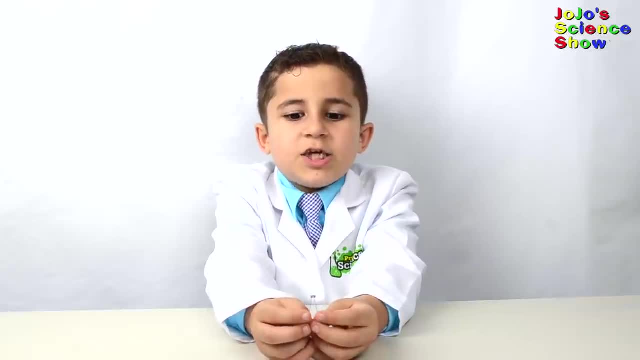 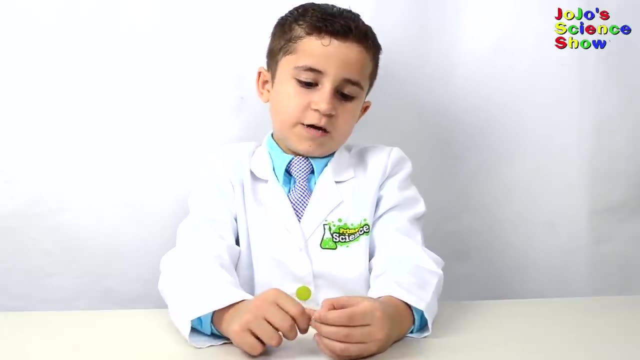 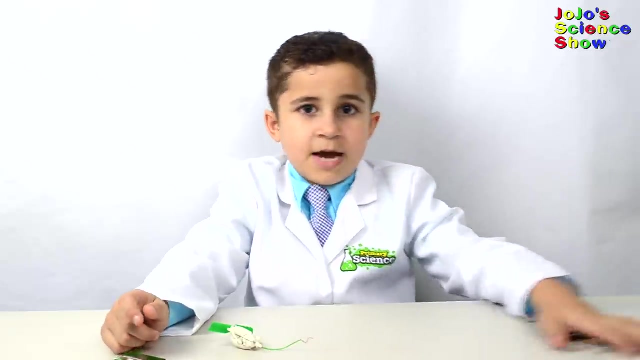 photoresistor conducts electricity when light is shining on it. It's like a gate that opens with light. When light hits here, then it allows electricity to flow. here You'll need a small electric motor and a battery, And to carry the electricity you'll need some alligator clips. 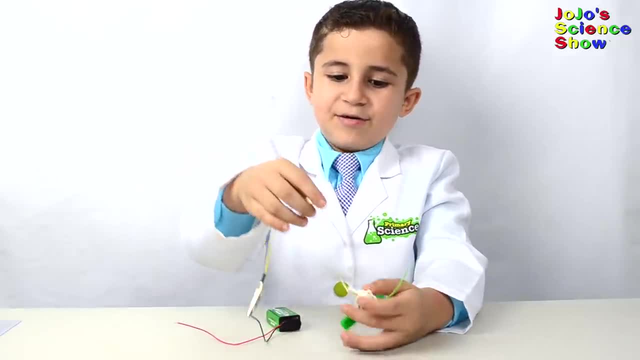 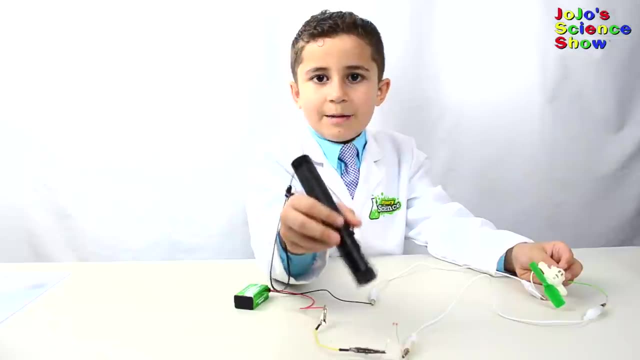 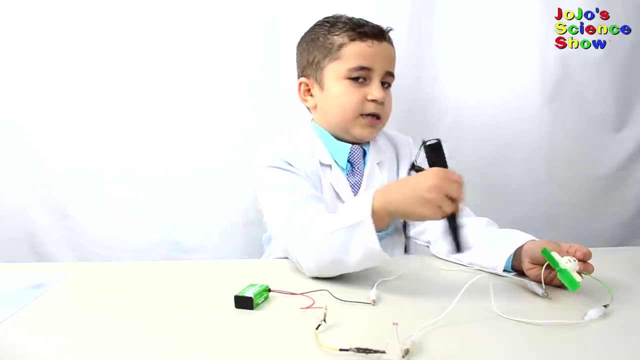 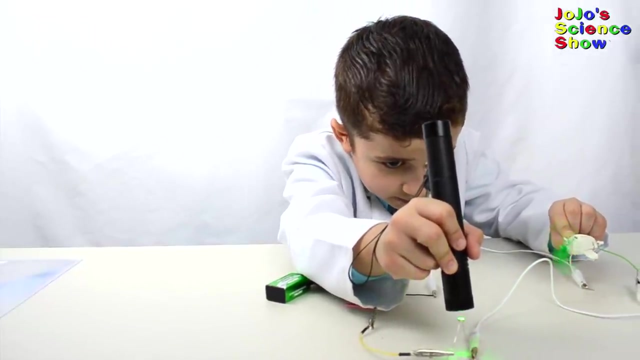 We built a circuit with the battery, with the motor and with the photoresistor. When I point the beam at the photoresistor, then it allows the electrons to flow from the battery to the motor and make it spin. See, When I shine on the photoresistor, the light allows the electrons to flow from the 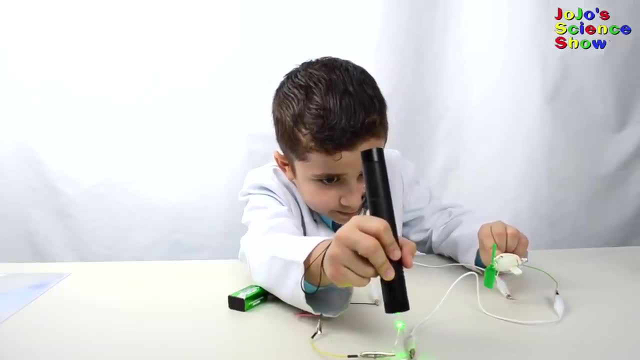 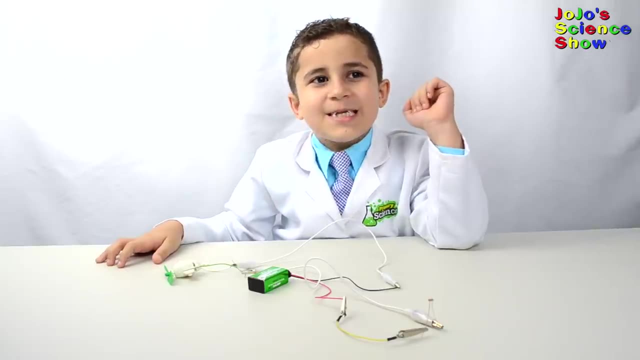 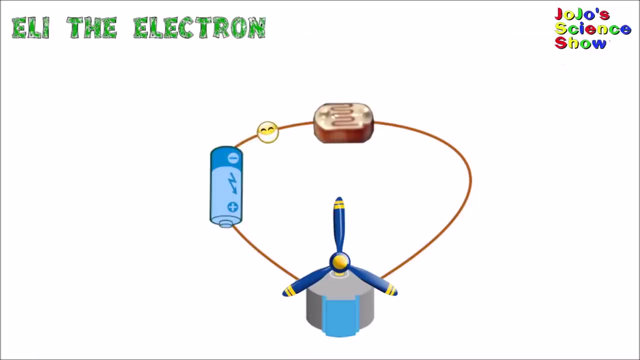 battery to the motor and then turns the reel Preparing for liftoff. We're gonna try it in the sun. Sunlight works just like the laser. Here's Eli, the electron, to show us how a photoresistor works, When the photoresistor's 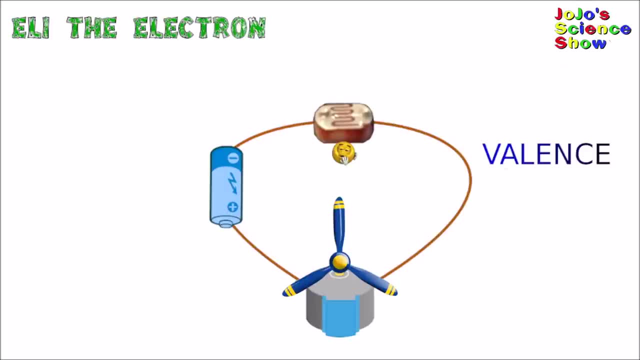 in the dark. Eli is tired and hanging out in the valence energy level. When he sees the light he gets excited and goes to the conduction energy level level And now he can move around the circuit. And he keeps moving as long as light is shining. 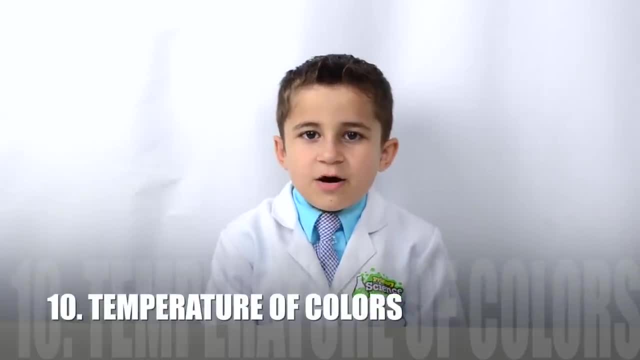 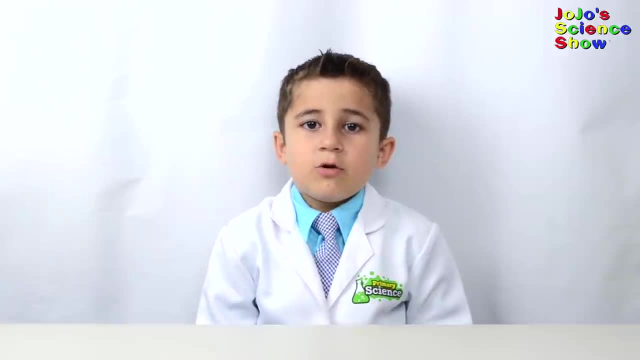 Vrooooom For this next experiment. we're going to measure the temperatures of different colors so that you know which colors address in different seasons. You'll be surprised of how big of a difference the color you're wearing makes A big difference For this. 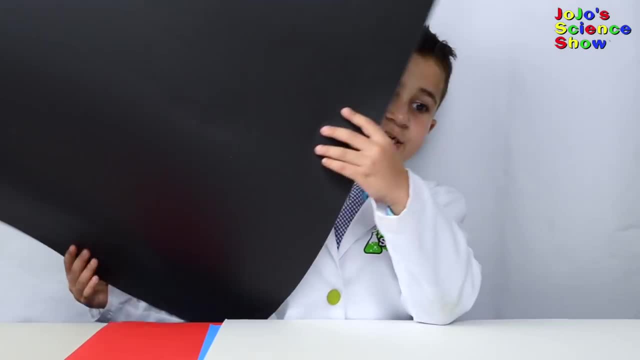 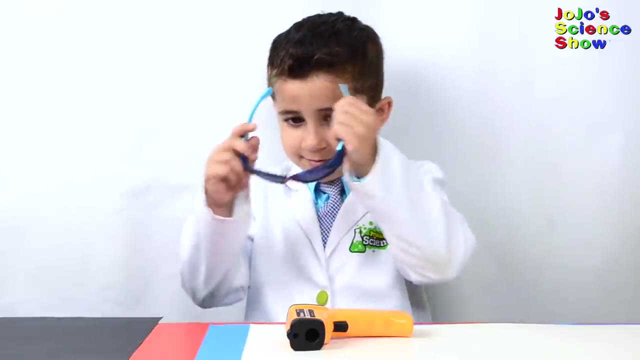 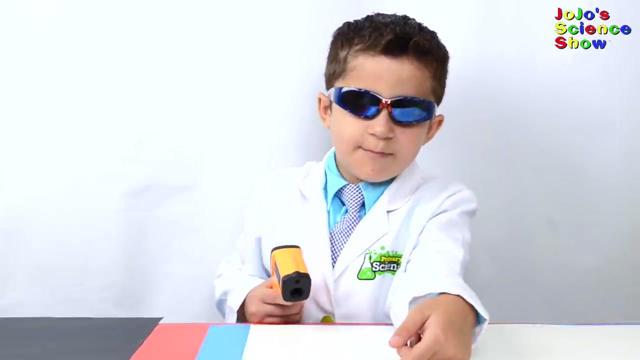 next experiment. you'll need four sheets of cardboard, each different colors. You'll need a white, a black, a blue and a red. You'll need some sunglasses and an infrared thermometer. Whenever you point it at something, that red dot measures the temperature of what's there. 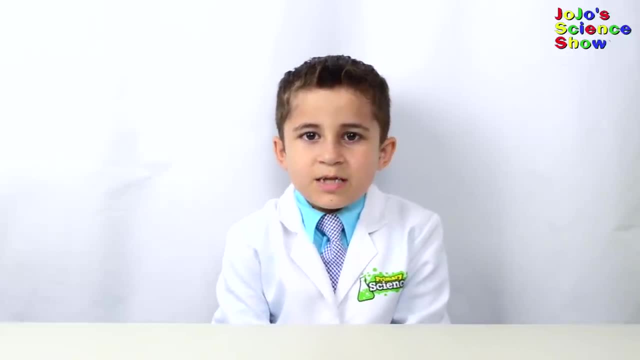 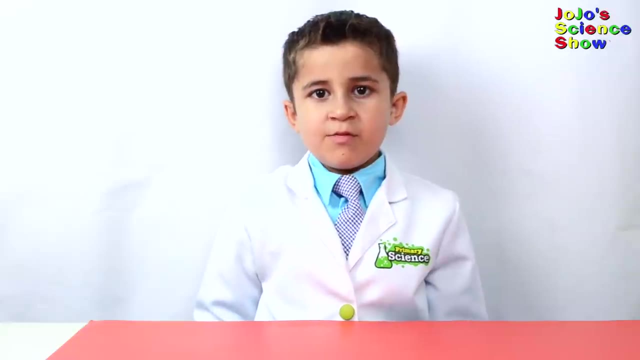 Do you know why objects have color? It's because they reflect light of that color and absorb all the other colors. Isn't that interesting? If you remember from our rainbow experiment, white light has all the colors of the rainbow. For instance, if you have a rainbow, it has all the colors of the rainbow. If you have, 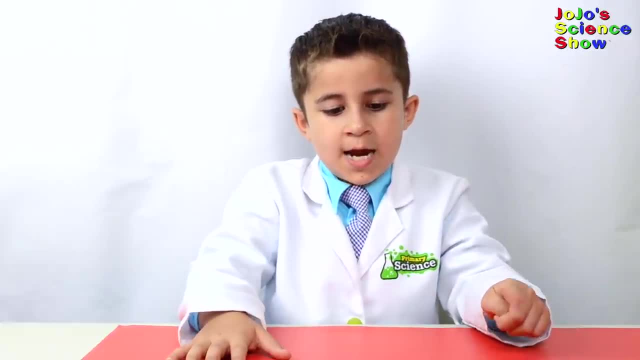 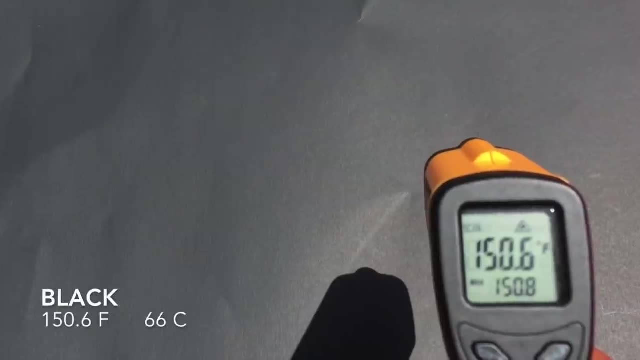 a rainbow, it has all the colors of the rainbow. If you have a rainbow, it has all the colors of the rainbow. For instance, this red cardboard reflects red light and absorbs the red. Let's check the difference in temperature between black and white. The black gets to 66 Celsius. 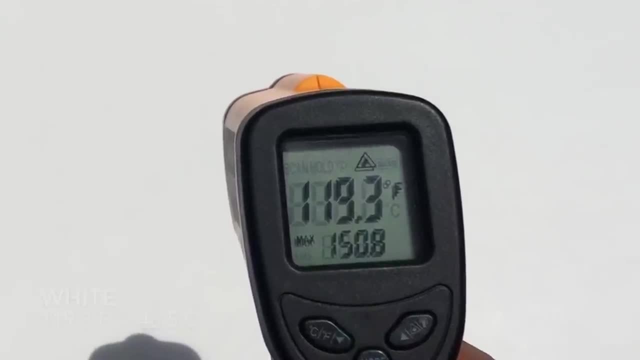 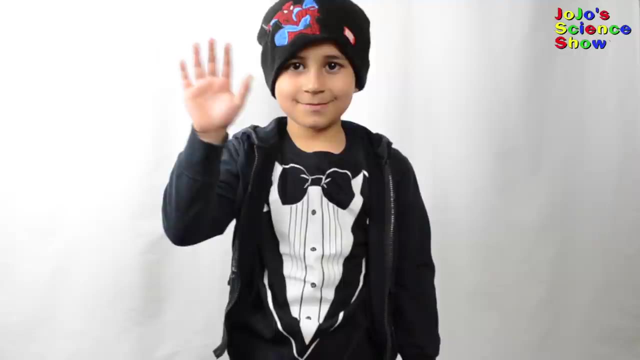 and the white only gets to 48 Celsius. That's about a 30 degrees Fahrenheit temperature difference. In the summer you should wear white clothes and in the winter you should wear dark clothes. Black absorbs all the colors of the light and will absorb all the colors. 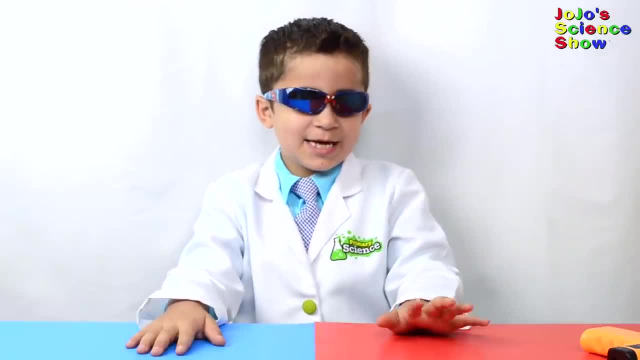 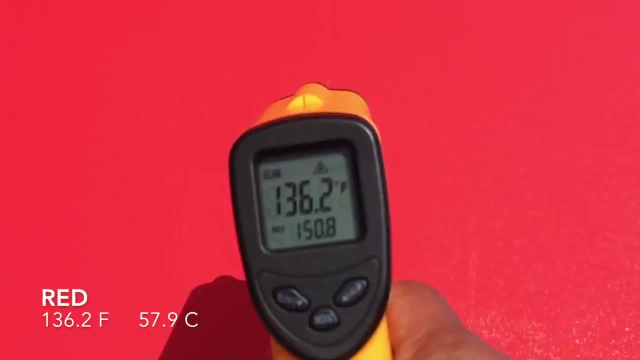 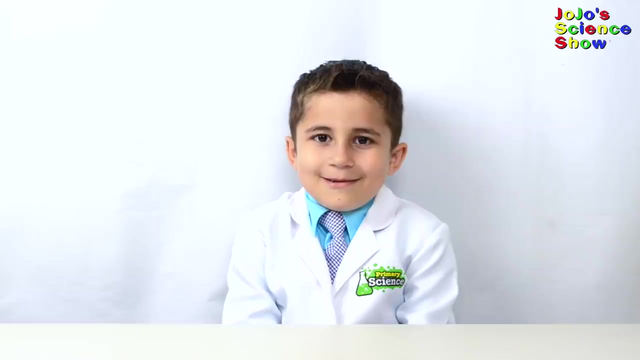 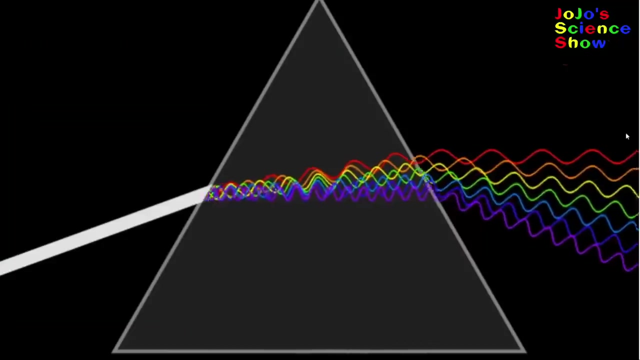 of the light. Oh Hi, Let's check the difference in temperature between blue and red in the sun. The red got to 57.9 Celsius and the blue was only 57.. Light is a wave that vibrates when it moves forward. Do you see how the blue light is vibrating faster than the red light? That's. 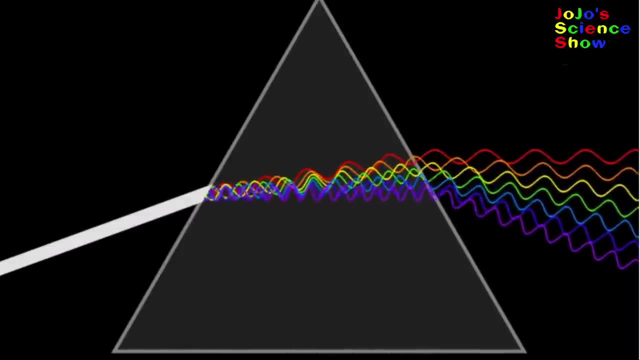 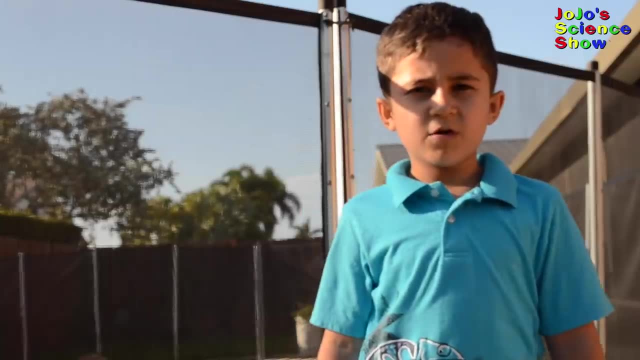 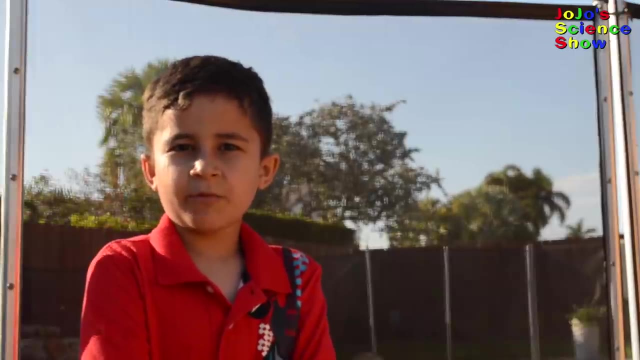 the blue light has more energy than the red light. Blue reflects the more energetic light, so it is slightly cooler than the red, and vice versa. The blue cardboard and this blue shirt are cooler The more energetic blue light is being reflected. The red cardboard and this red shirt are both.